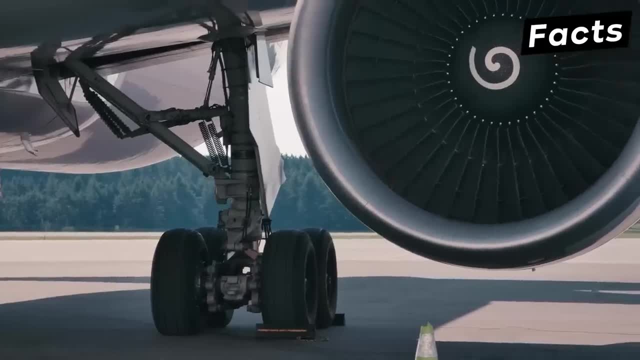 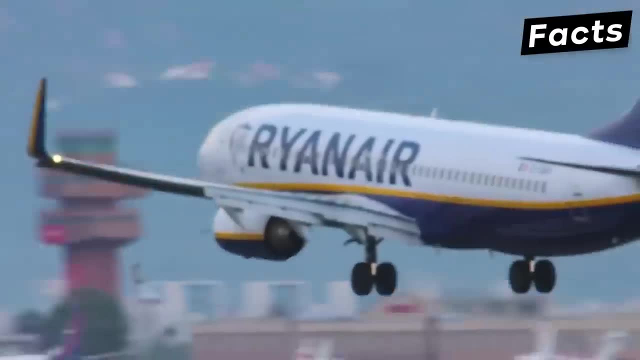 engine shutdown, Because engines are so well engineered and built. bird strikes rarely cause fatalities Well, except to the bird. However, it's been shown that a bird strike can still take down a plane. Because of that, this test is possibly one of the most important ones. an 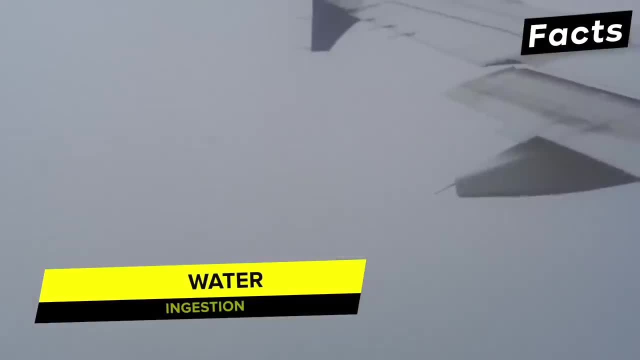 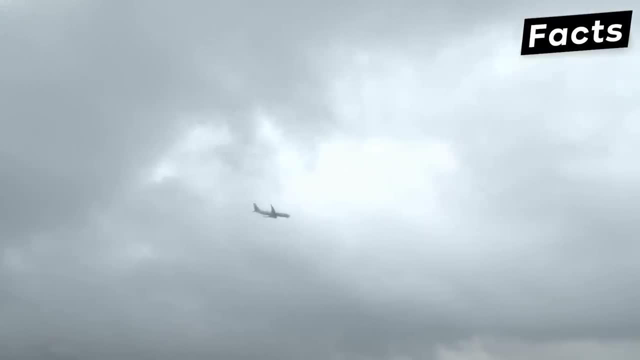 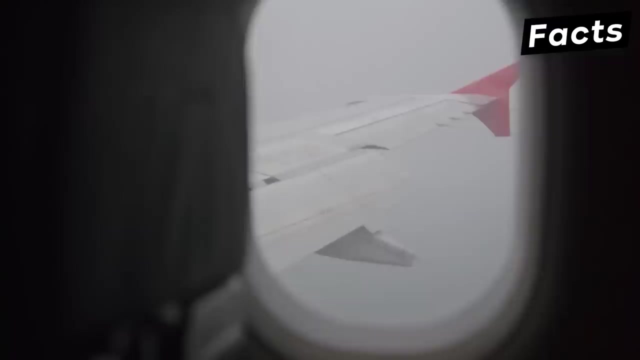 aircraft engine needs to go through Each day. aircraft engines are exposed to extreme weather conditions and oftentimes they're forced to operate through rain and storms. The exposure to water in the skies means that each engine has to be able to function properly during such conditions. They need to be able to take in 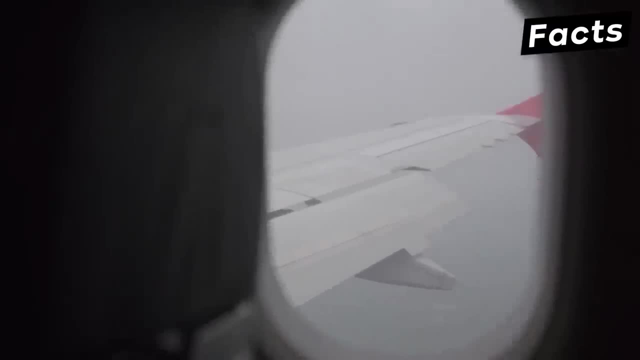 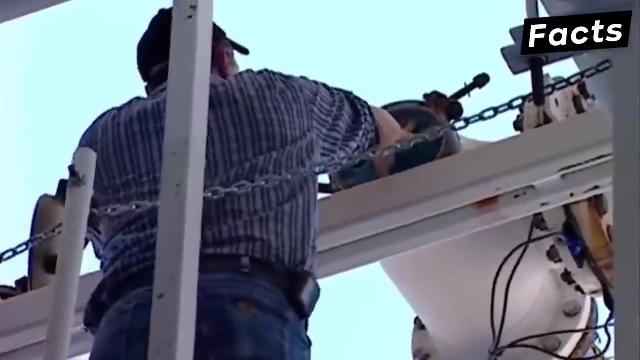 large amounts of water. so to test engines for how capable they are, water ingestions tests are a must. Manufacturers do these tests by forcing a stream of water into running engines. They fire up to 800 gallons of water every day, and they're able to take in as many as 800 gallons of water. 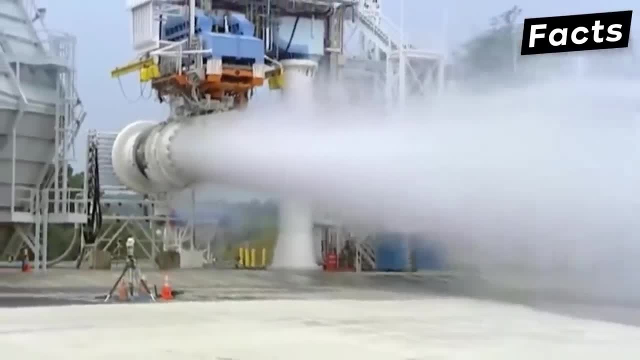 per day. They're able to take in as many as 800 gallons of water per day, and they're able to take in as many as 800 gallons of water per minute into the engine. When this test is conducted, the goal is to have the water pass through the engine and be shot out the back without reducing 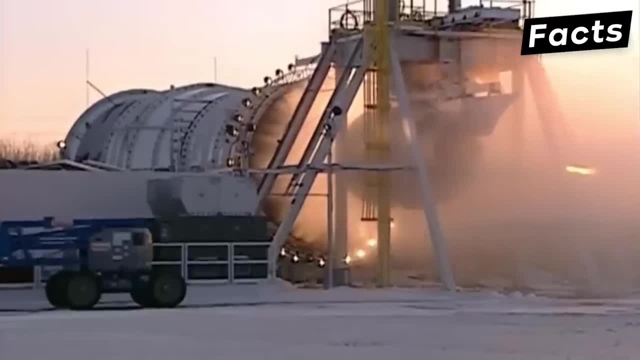 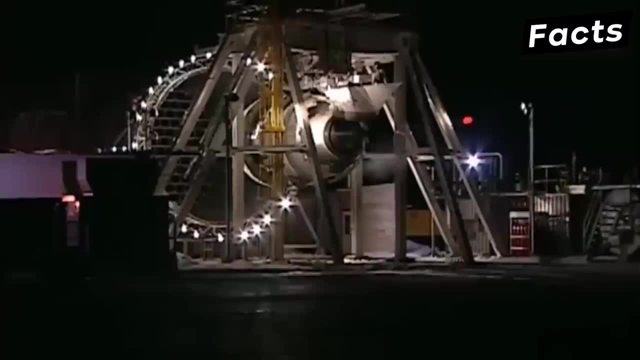 thrust. If the test is a success, it means that the engine can handle the forecast rainstorms and run through pools of water. Alongside this test, the engines are also put through a wind test. Crosswinds can make the aircraft lose its direction, making it almost impossible to land. 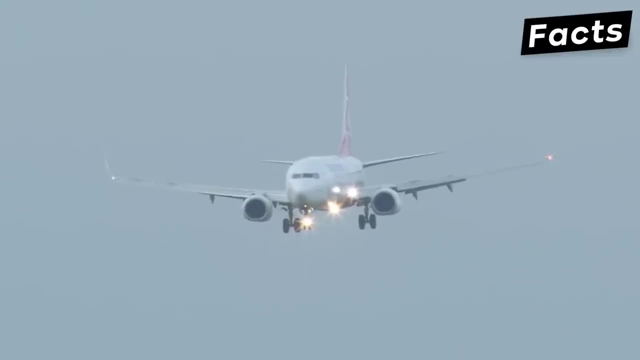 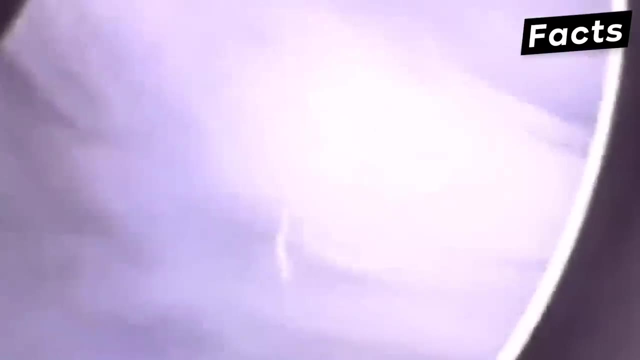 or take off. In addition, crosswinds can also cause turbulence, making the engine fan blades vibrate, causing damage to the blades. To avoid this, wind tests are conducted where the air is forced through the engine at high speed and several blast-simulated crosswinds are forced. 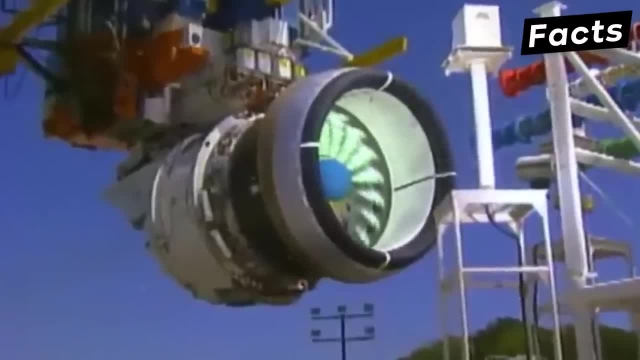 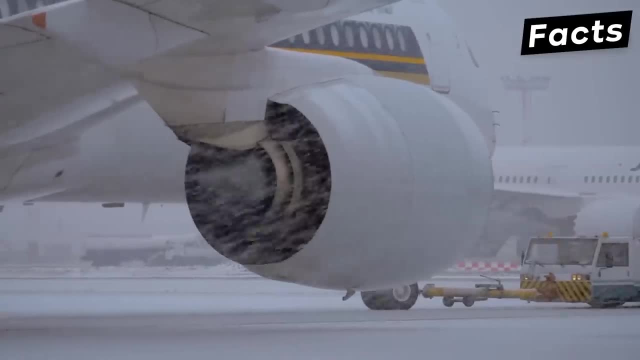 across it, measuring its ability to withstand the strongest of gusts. Although water and wind might be a concern for the engines, it doesn't come close to fire and ice Freezing temperatures can be a huge problem for an engine, especially if the engine isn't tested against these conditions. 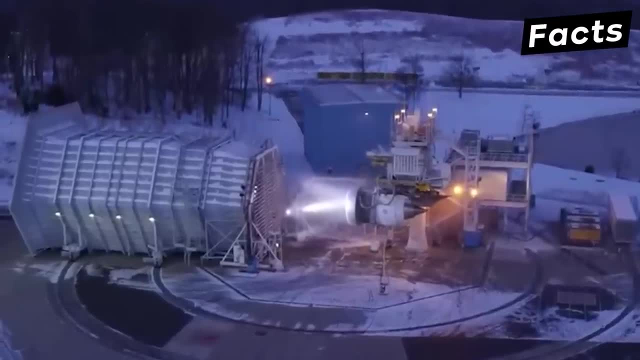 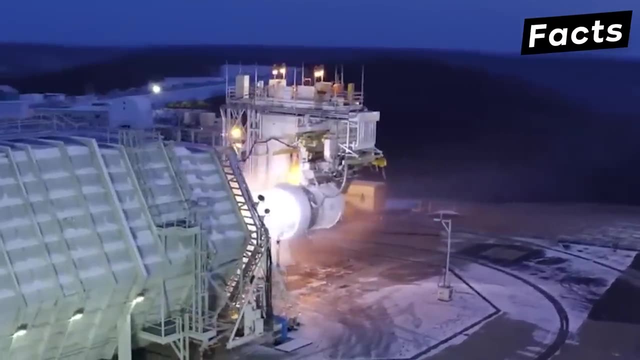 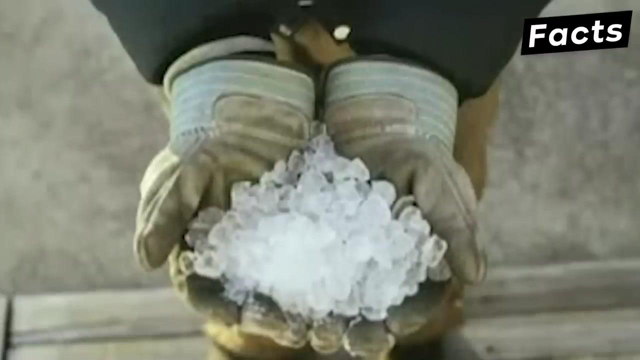 One of the ways this concern is tested is by placing the engine in an environment where the temperatures are cold, allowing the engine to spend days or weeks there and testing how it operates in that temperature. Another way to test the engine against ice is by shooting ice into a running engine. These big balls of hard. 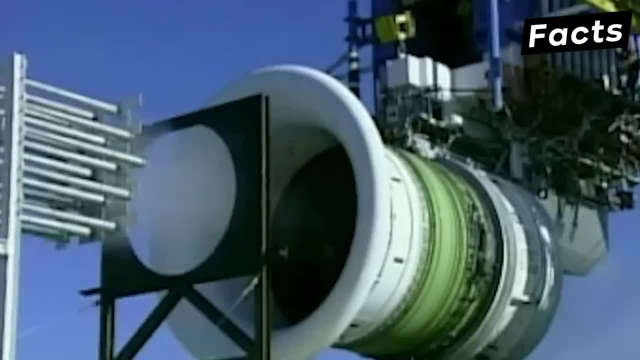 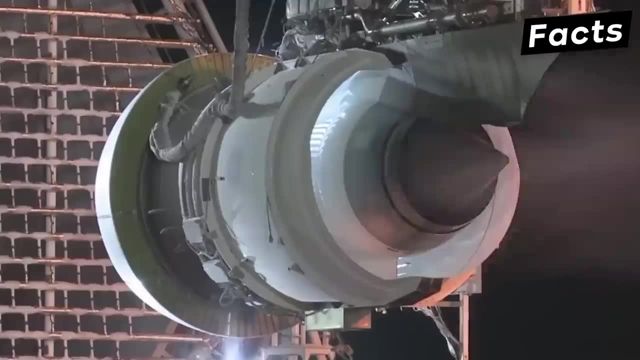 compacted ice are set to mimic the effects of flying through a hailstorm. This way, manufacturers can determine whether the engine will be damaged from the ice or whether it is able to ingest the ice and continue operating When it comes to fire and extremely hot temperatures. 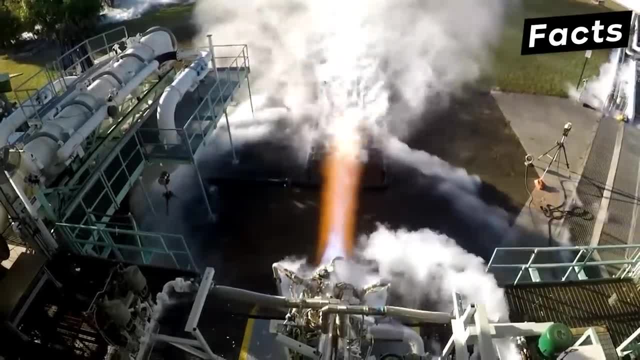 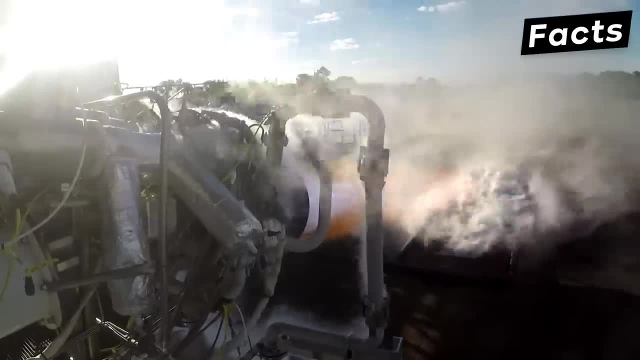 the manufacturers have the same type of tests as the ice tests. The engine is placed under a huge amount of heat. Engineers will then run the engine at maximum temperature for extended periods. Just like ice can be an issue, so can fire. These engines can be designed to withstand. 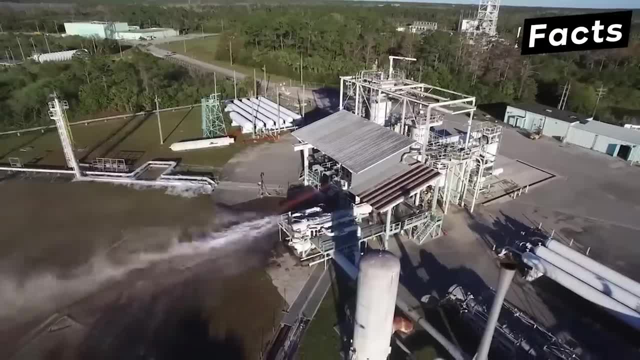 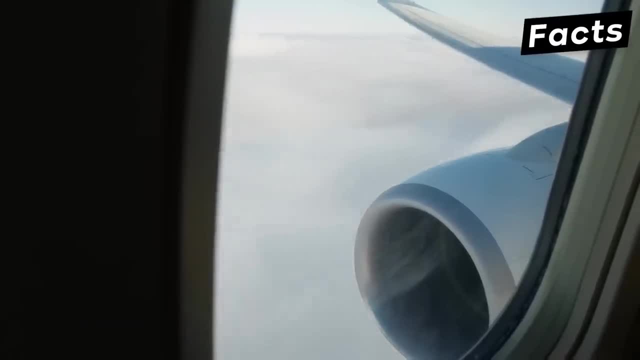 some of the most extreme weather conditions and anything that comes their way. An aircraft engine must perform safely in high altitudes. If an engine isn't designed well, it may fail to operate at such altitudes, causing a situation that is not well-prepared. 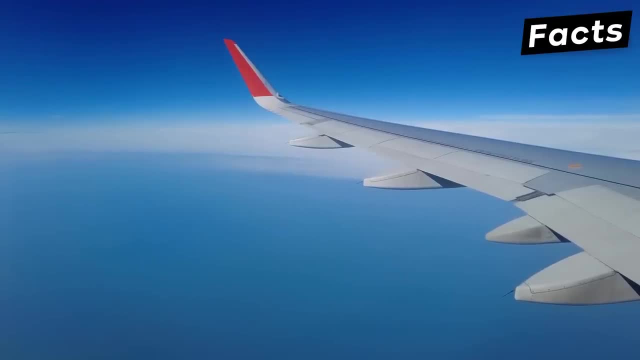 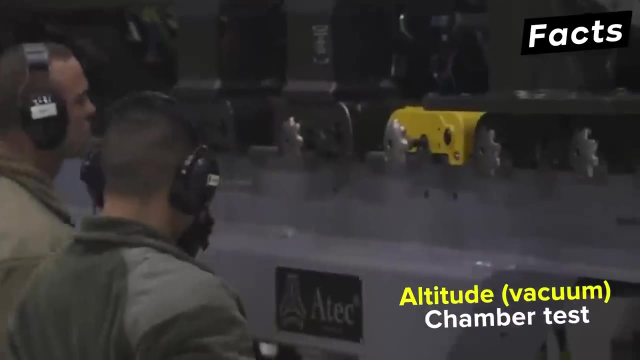 series of failures throughout its lifespan. Due to this, each engine is tested on the ground in an environment simulating the required altitudes. This test, also known as the altitude or vacuum chamber test, is conducted in a vacuum pressure vessel in which the engine is tested against high 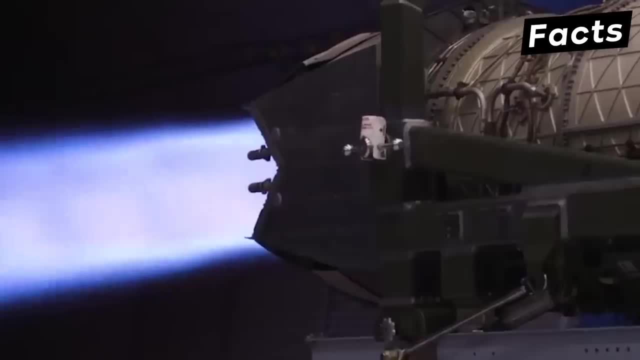 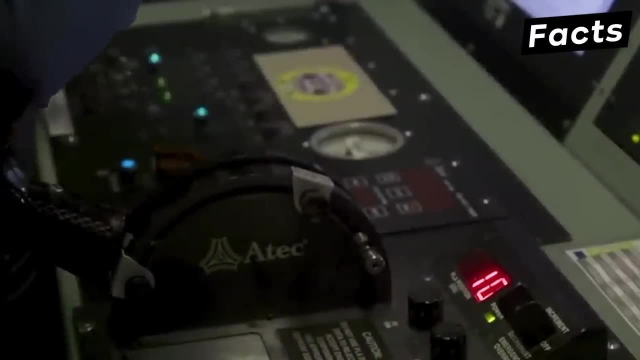 altitude flight conditions. The chamber has all the equipment to mimic the atmospheric pressure at such altitudes. The altitude inside the chamber is set by pumping down the chamber to the lower atmospheric static pressure for the specified altitude, And then the Mach number is set by. 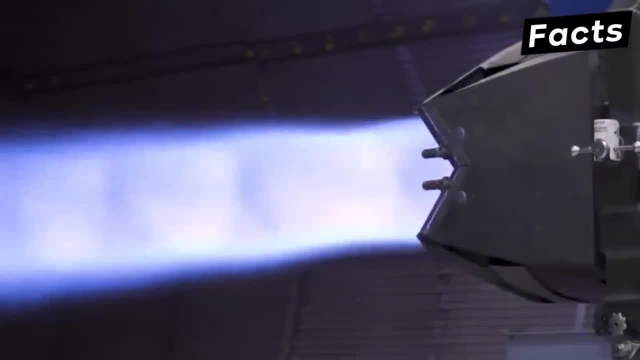 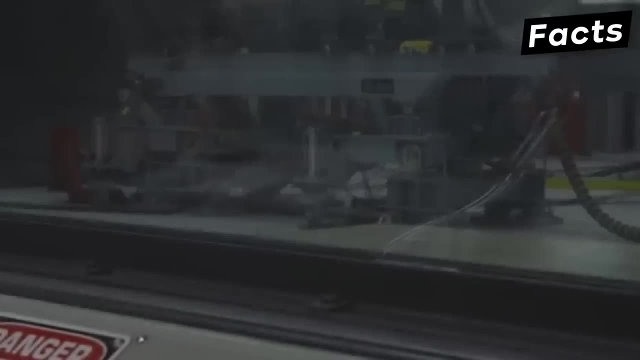 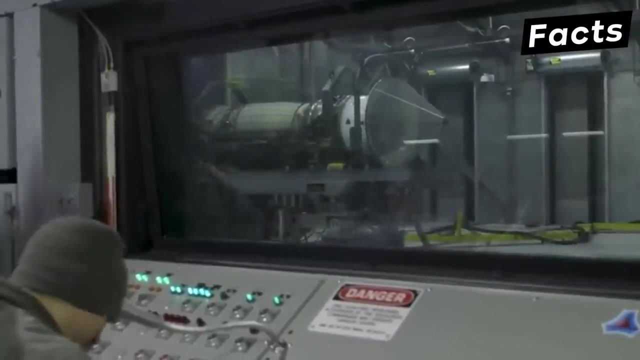 supplying air at the proper total pressure and total temperature to the engine inlet. This test is conducted so that manufacturers can determine how the engine performs under these conditions. If everything goes smoothly, the engine is ready to go through to the next test. But if there's the slightest concern during the test, manufacturers will have to go back and make. 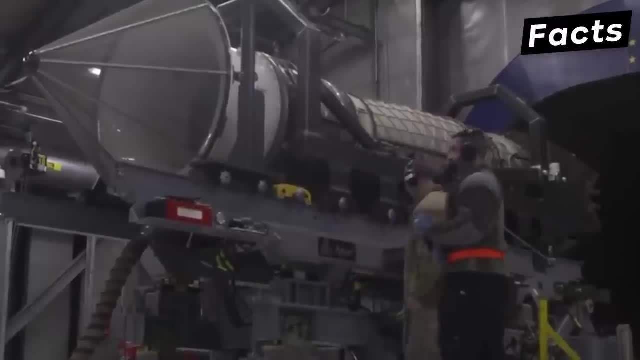 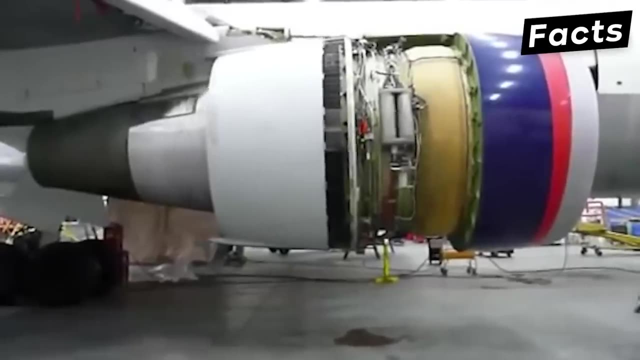 any necessary modifications to the engine to make sure that it'll operate as planned at such high altitudes. The engine's ability to produce reverse thrust is used to slow down the aircraft during landing. This is a key component of every engine that allows it to. 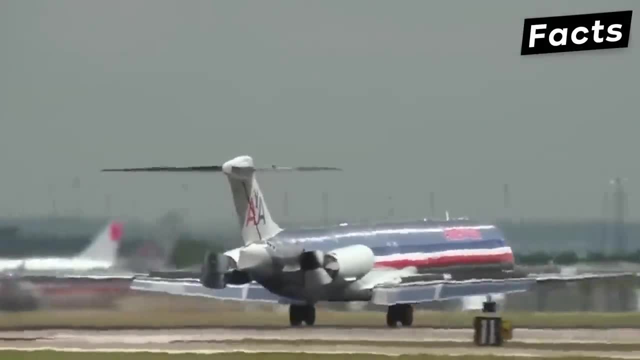 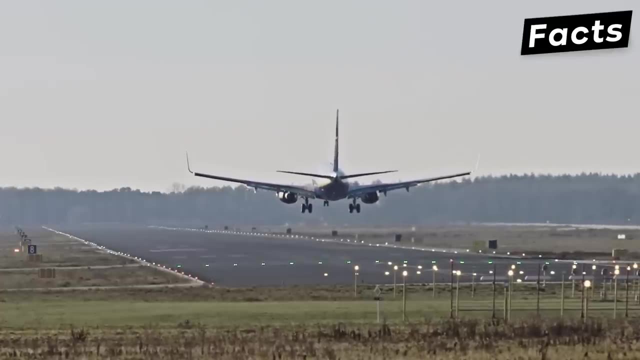 slow down to the desired speed when it's time to land the aircraft. Without this, airplanes wouldn't be able to make safe landings, resulting in many disastrous situations. So it's become a must for each engine to be tested for thrust reversal. This test is intended to appraise the safe operating. 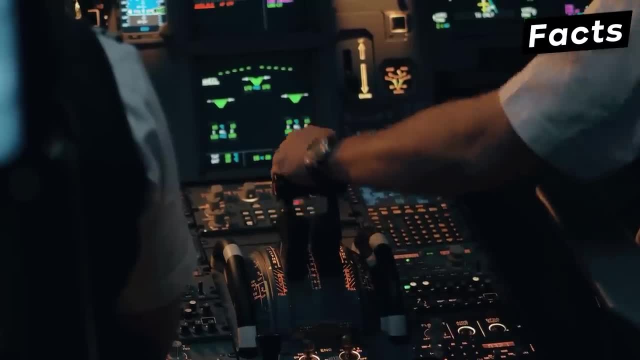 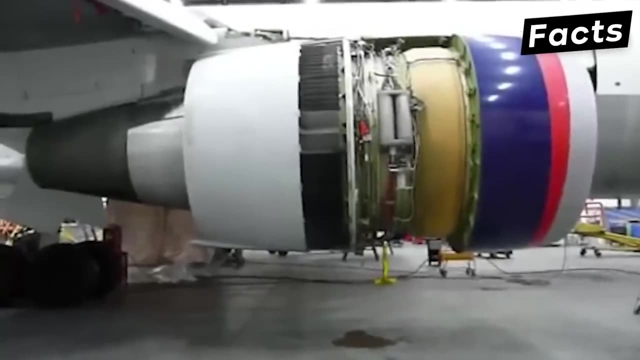 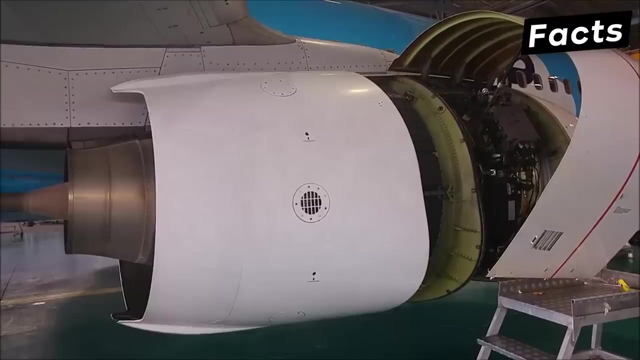 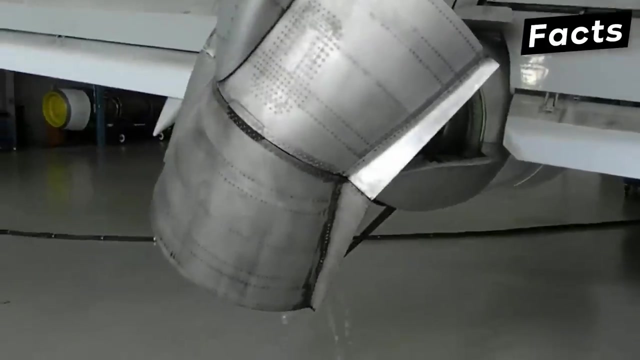 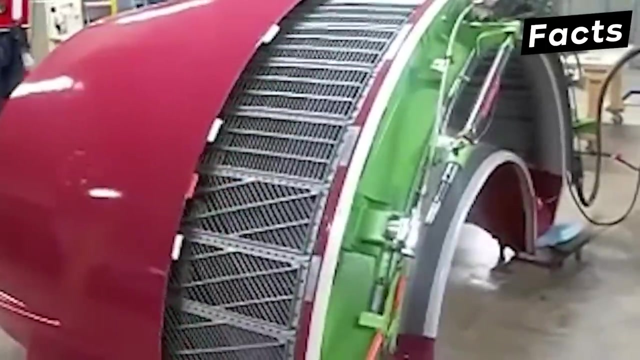 conditions and establish the engine's stall mark. The test is intended to appraise the safe operating conditions and establish the engine's stall mark. The second part of the test would consist in a test for level prophetic renders. This is what happens when some aircraft ajusts themselves over time. 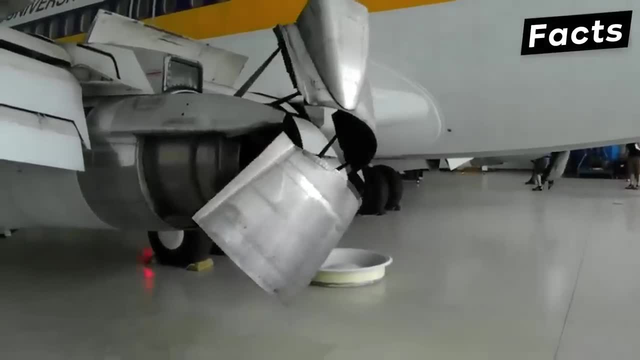 This is how the sausageixed engine is tested. during landing, The thrust reversers are engaged. This is occurred when the thrust reversers engaged. This test is conducted in a full 1972 air tunnel where the aircraft landing is simulated, while the, as most of them, have been produced with safety measures to prevent that from happening. 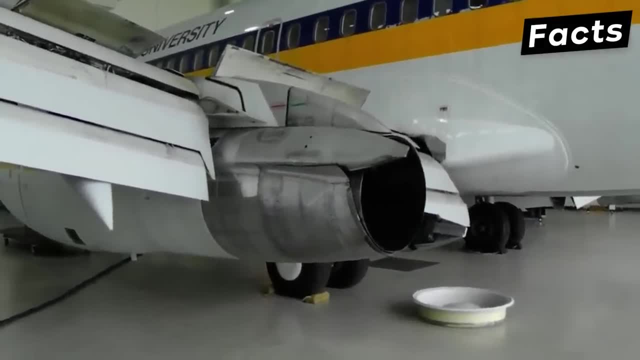 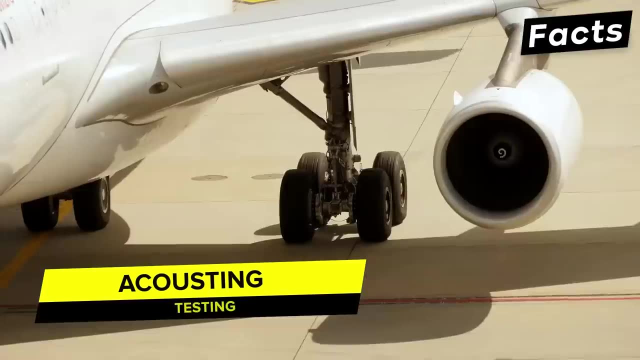 However, they still go through these tests as a way to ensure the manufacturers that the engines can perform in reverse thrust, thus helping the aircraft land safely. We're not going to lie: aircraft engines are loud, But compared to the engines used 20 years ago, we can safely say that they've become increasingly quieter. Many manufacturers have set a goal to make their engines as quiet as they can be, and by 2050 it's said that engines will have reduced their noise by 65% If you put an engine inside a building as it's running at full power. 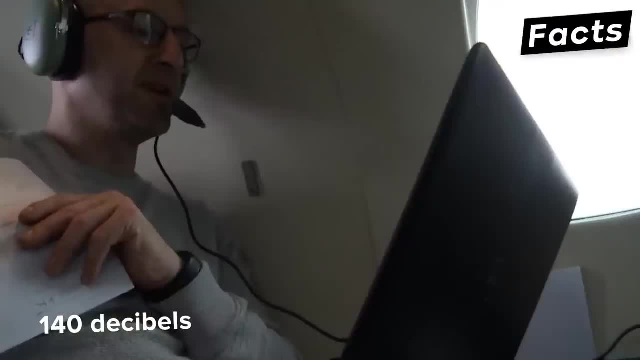 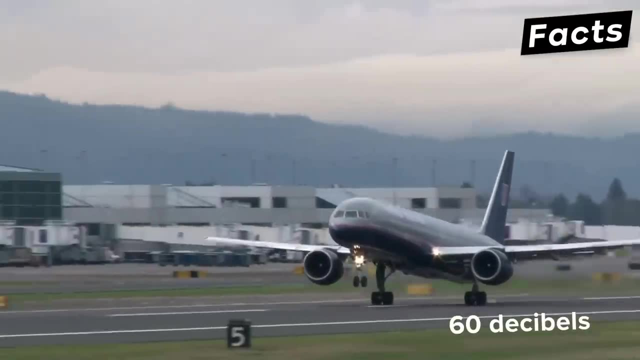 you'll get a noise level of 140 decibels, which is painful to any human being. But when that same engine runs at full power outside, the noise levels are within 60 decibels, well within the environmental requirements. There are tough regulations on aircraft noise. 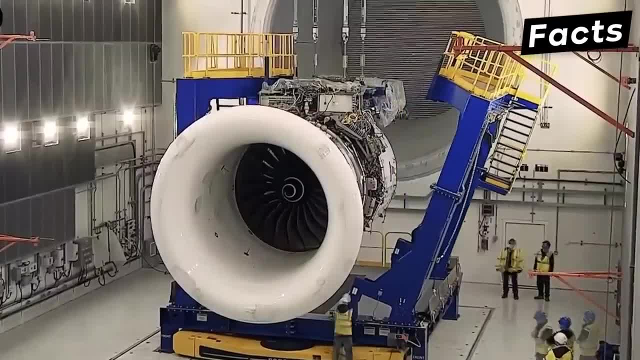 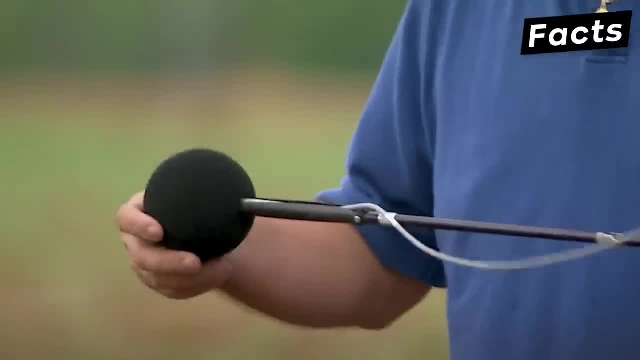 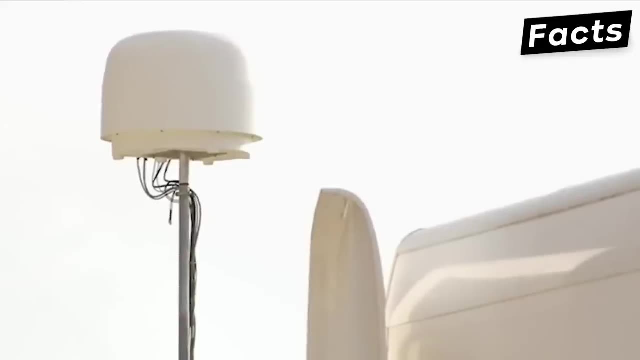 so each manufacturer has to precisely measure their engine's sound level. This is done by placing the engine outside, where incredibly sensitive microphones are placed around the engine test bed and can detect changes in the noise to within a fraction of a decibel. The engine operates from low to maximum power to gather every noise the engine makes. 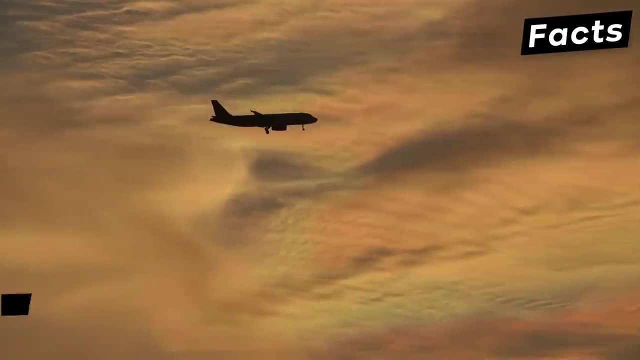 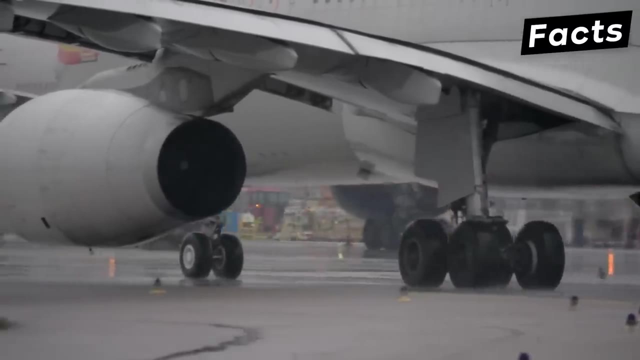 An aircraft engine has to go through the test flight or the various tests in the sky. Most of the tests are conducted on the ground, but as soon as the engine passes them, it's time to take it to the sky and see if the engine will operate as expected. 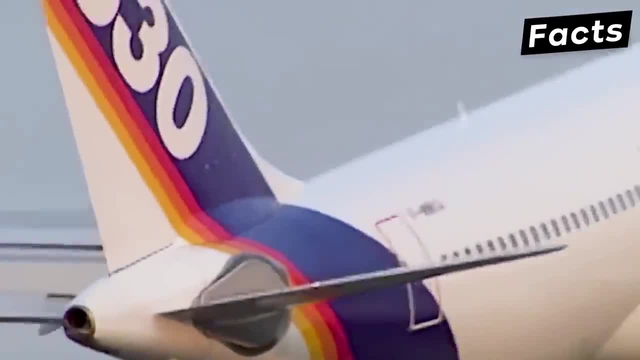 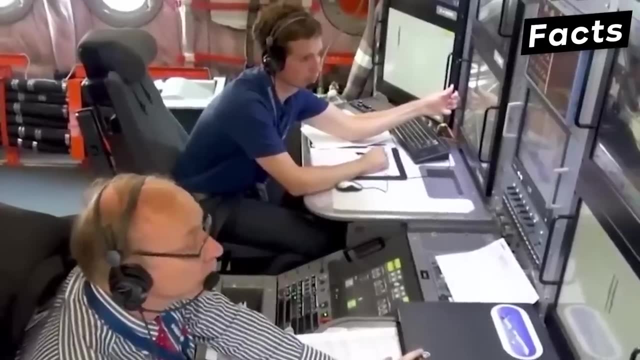 This way, the engine's reliability is truly tested. Before an engine takes to the sky, it has to be certified as safe and fit for flying. Part of that certification process is taking the engines into the air, and for that modified aircraft known as test beds are used. 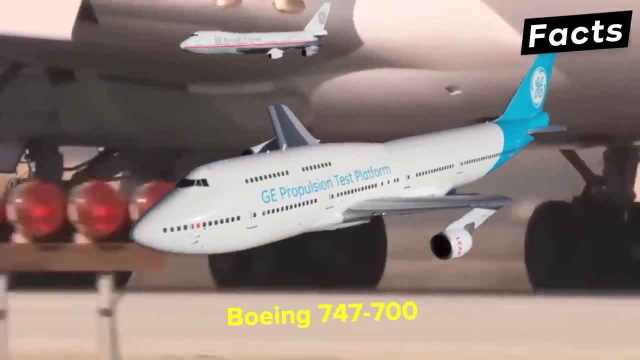 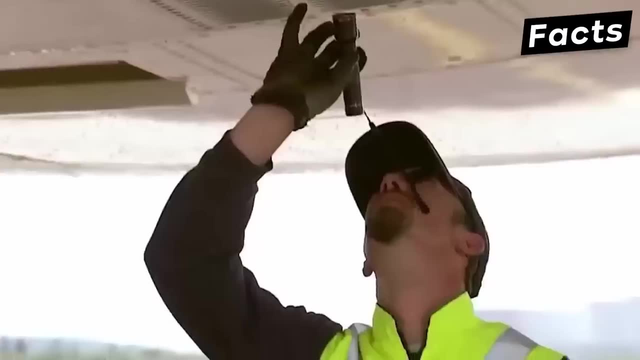 One example is GE's flying test bed, the Boeing 747-700,, which carries test engines. The variety of test beds is endless, but they all have the same goal: They need to take the engine to the sky and allow it to show what it's capable of.